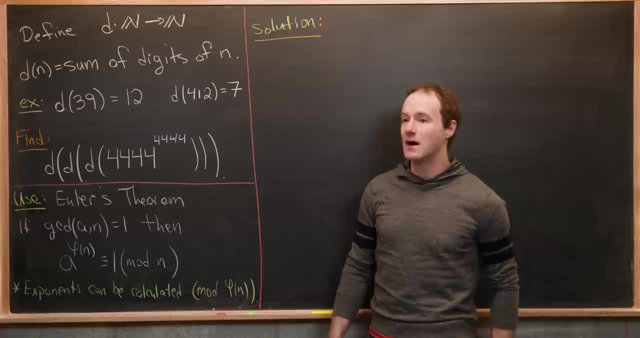 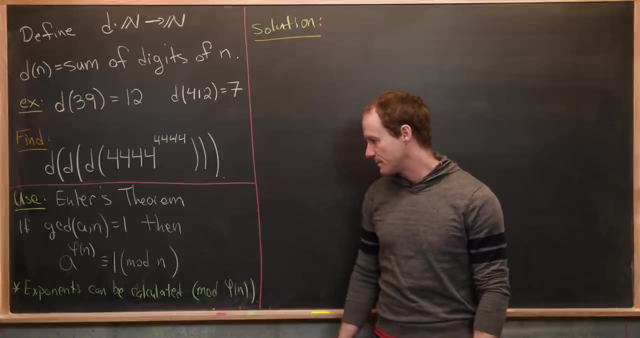 is Euler's totient function And that counts the number of numbers between 1 and n that are relatively prime to n. And the takeaway from Euler's theorem is that if you're working with a congruence, the f of n is the number of numbers between 1 and n that are relatively prime to n. 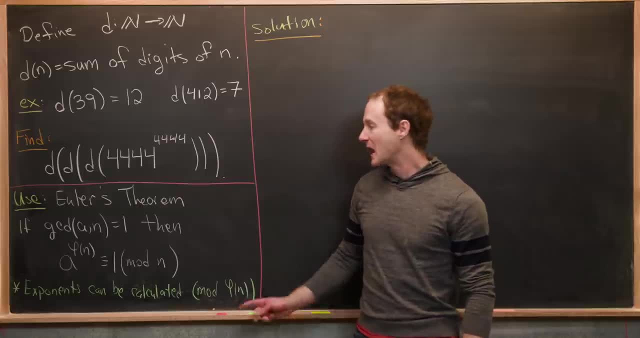 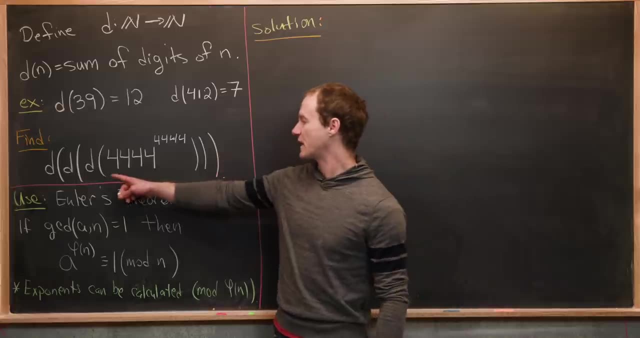 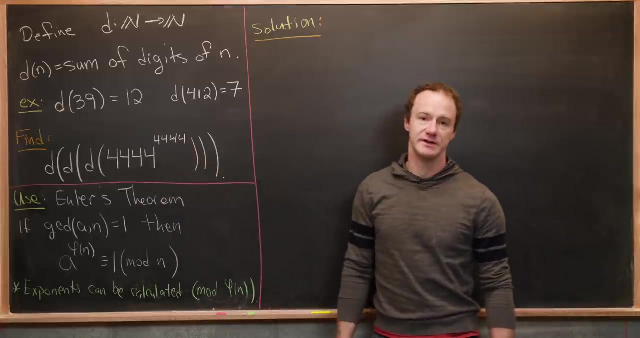 The exponents can be calculated mod phi of n, as long as the base is relatively prime to n. So let's first, instead of calculating anything to do with the digit sum, let's see if we can calculate what this is congruent to mod 9.. And why mod 9?? Well, that's. 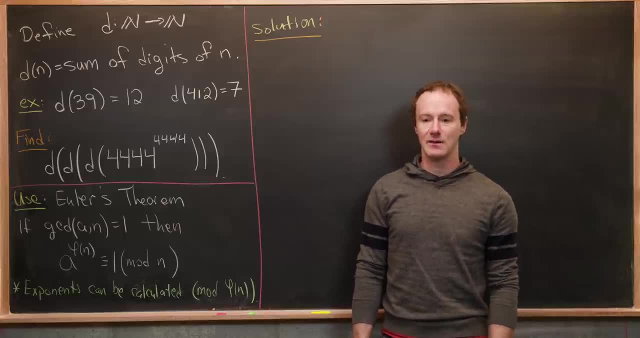 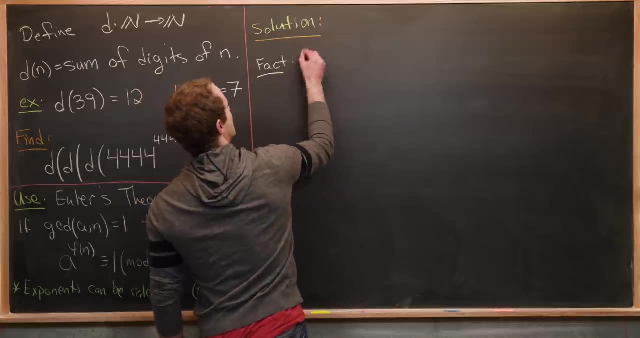 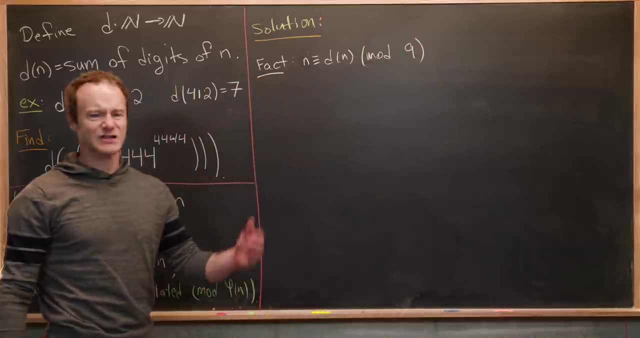 because the digit sum of a number and the number are congruent mod 9.. So let's maybe write that real quickly as a fact, Euler's generalization of Fermat's little theorem- And we're going to write that n is congruent to the digit sum of n modulo 9.. And that's actually pretty easy to see. 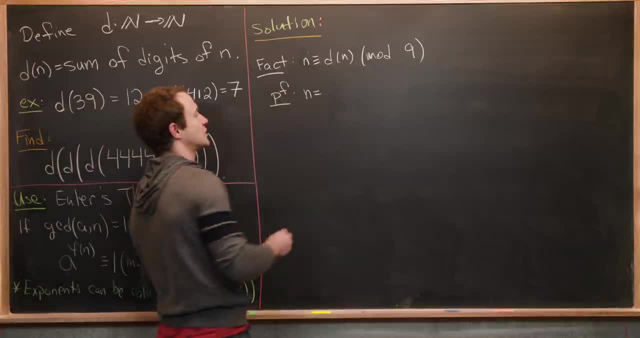 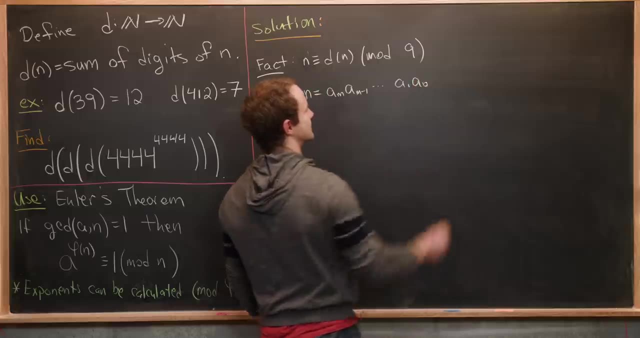 so we'll do a little sketch of a proof here. So I'll write it in terms of digits, as a sub m, a sub m minus 1, all the way down to a sub 1, a sub 0.. Now expanding this with powers of 10. 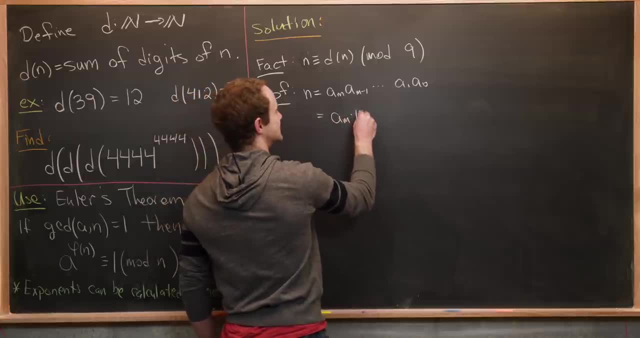 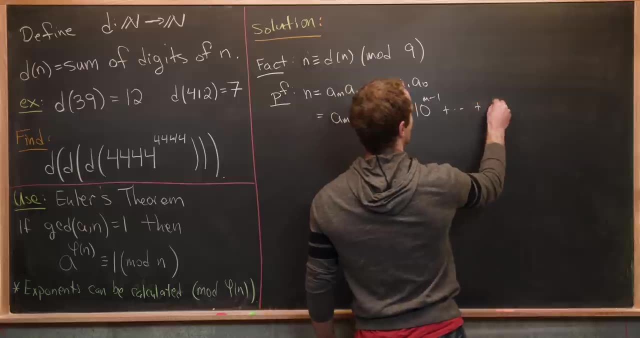 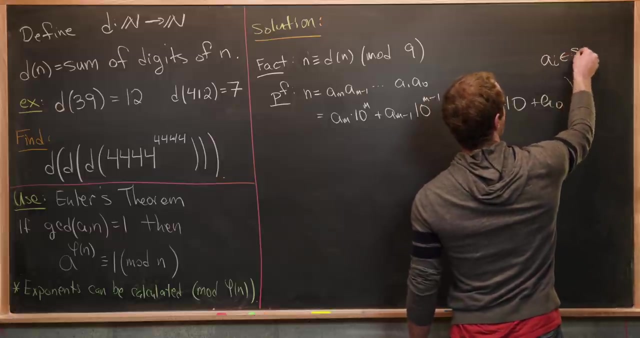 we see that this is a sub m times 10 to the m, Plus a sub m minus 1 times 10 to the m minus 1.. Plus all the way down to a sub 1 times 10 plus a sub 0.. And the important thing here is that all of these ai's are on the set 0 to 9.. 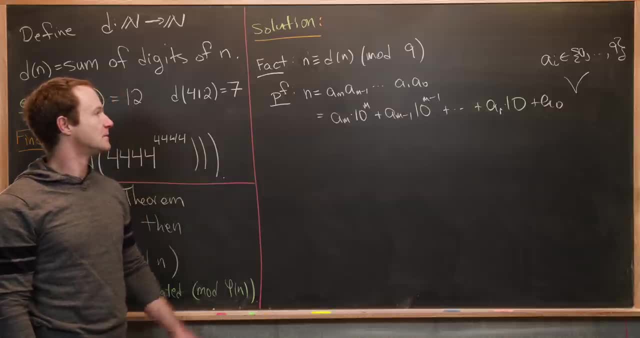 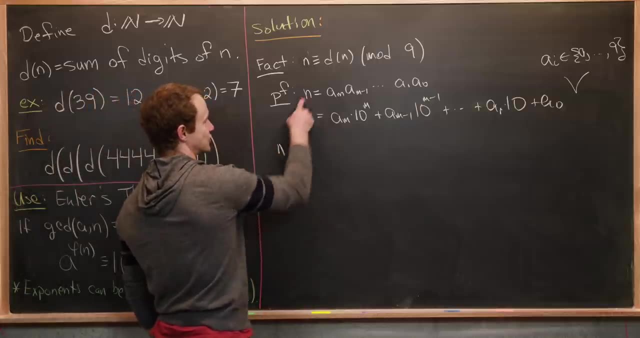 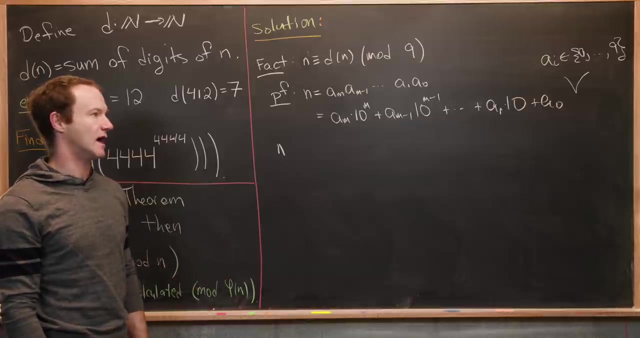 Because they make up the digits base 10 of n. Now we'll reduce both sides of this modulo n And notice that if we reduce this side we'll just get the n, And if we reduce the right hand side, every power of 10 is congruent to 1 mod 9.. 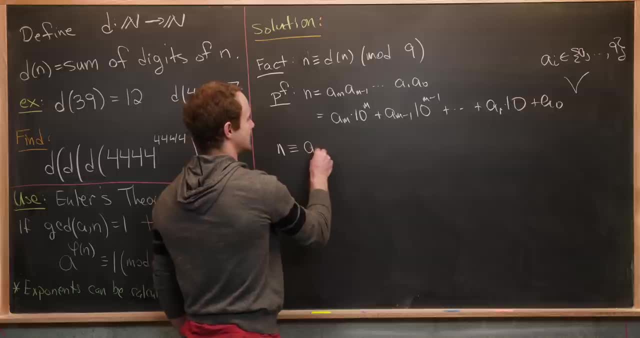 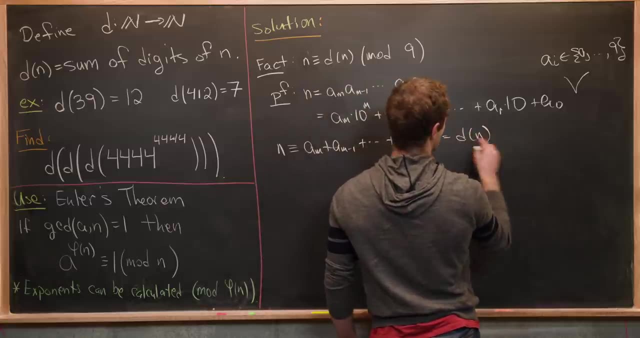 That's pretty easy to see. but that makes this equal to a sub m plus a sub m minus 1, all the way down to a sub 1 plus a sub 0. but that's exactly d sub n modulo 9, which is exactly what we wanted to. 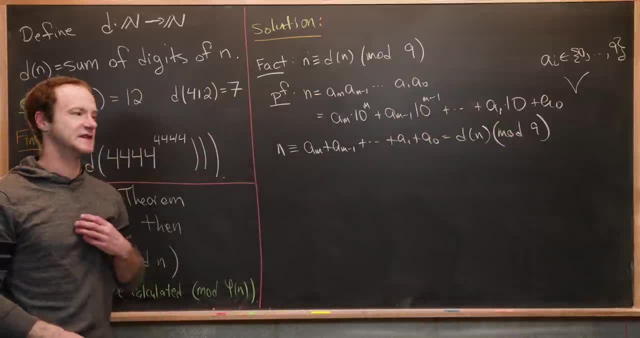 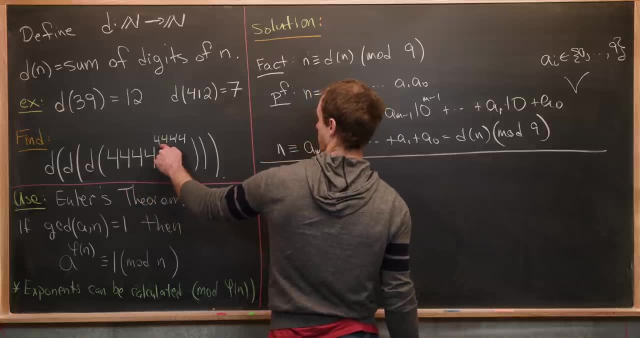 show. So now that we've got our motivation for why we should look at this mod 9 in the first place, let's go ahead and calculate 4, 4, 4, 4 to the 4, 4, 4, 4 mod 9.. And if we know what that is- mod 9, then we know what the 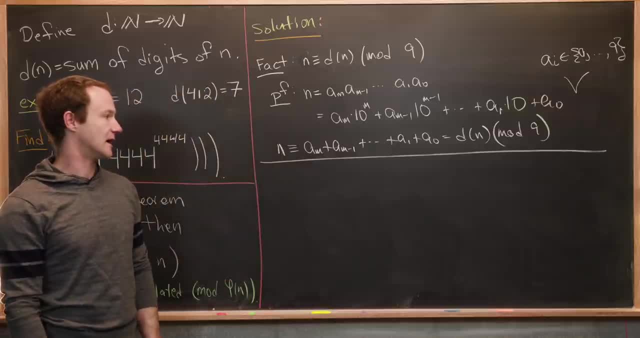 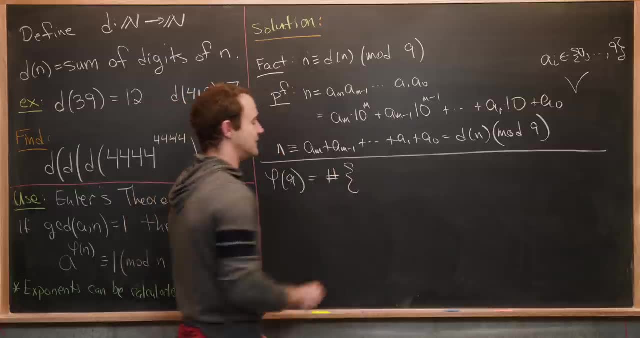 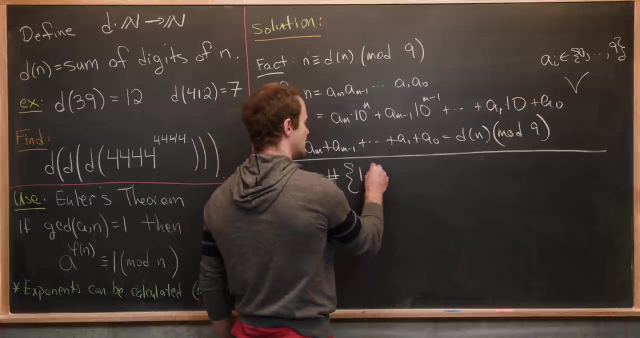 applications of these digit sums to that number is mod 9.. So, first off, I want to notice that phi of 9.. Well, like I said, that's the number of numbers between 1 and 9 that are relatively prime to 9.. So in this case we get 1,, 2,. 3 is not in there, but 4 and 5 are in there. 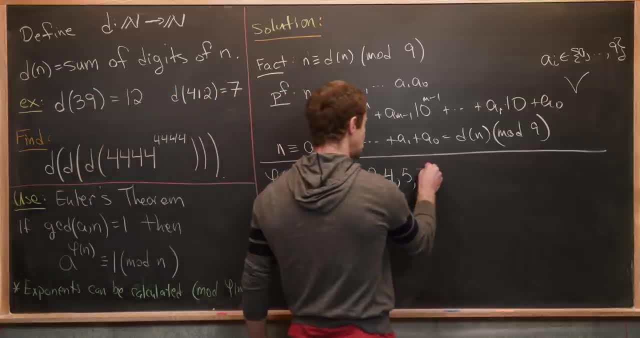 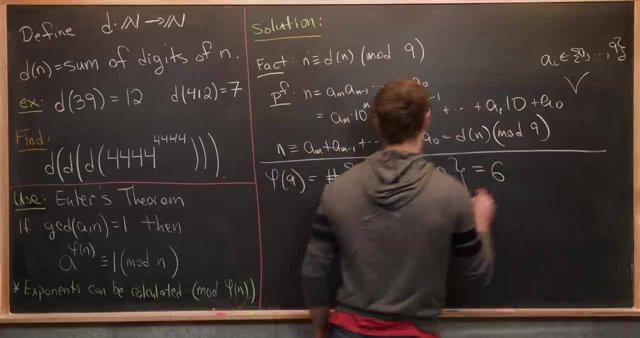 6 is not in there because they have a GCD of 3, but 7 and 8 are in there. So notice, we get 6 total numbers. So that means phi of 9 is equal to 6.. Now we're going to perform division with. 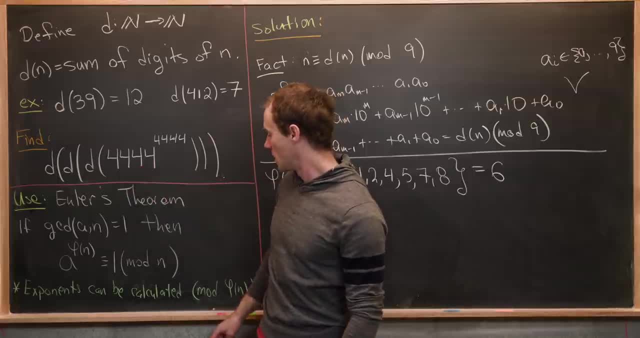 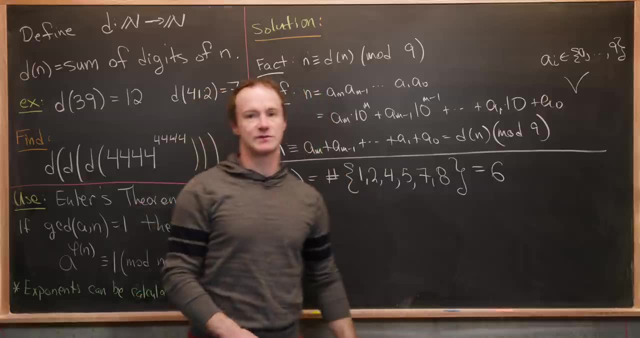 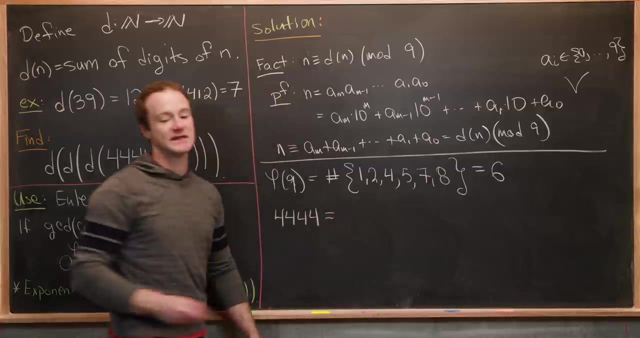 remainder of 4, 4,, 4, 4 with 9 as the divisor And phi of 9 or 6 is the divisor, And then use Euler's theorem to reduce this modulo 9.. So I'll just write that calculation down: We have 4, 4, 4, 4 is equal to 9 times 4,. 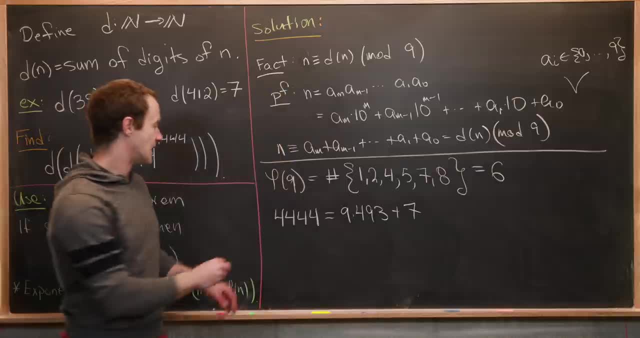 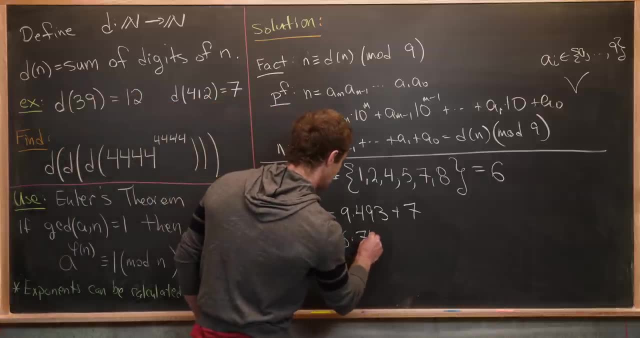 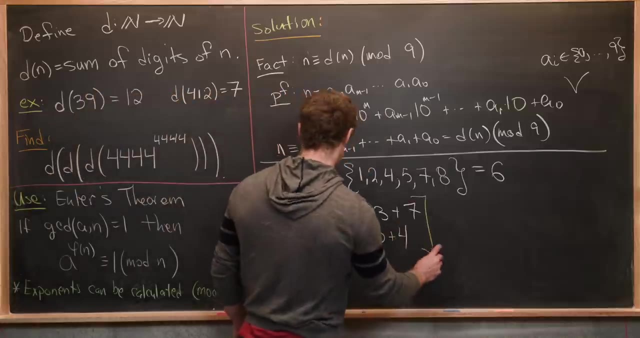 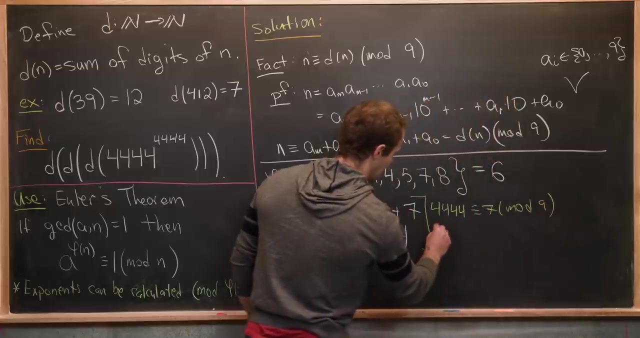 9, 3 plus 7.. And then 4, 4, 4, 4 is equal to 6 times 7, 40 plus 4.. But now let's recall that that is equivalent to saying that 4, 4, 4, 4 is congruent to 7 mod 9.. And that 4,. 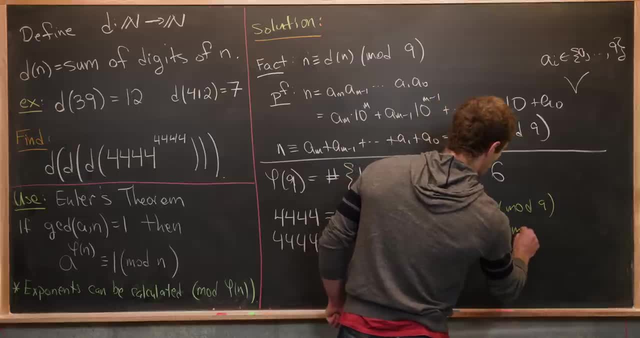 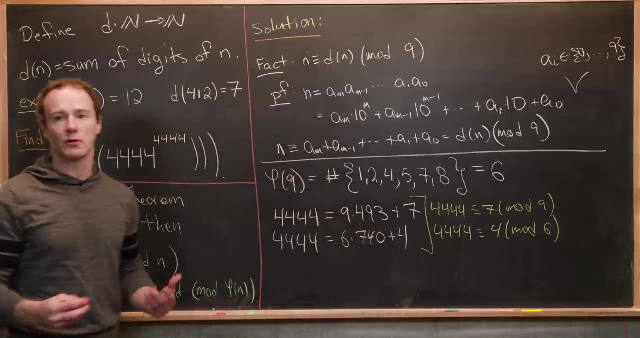 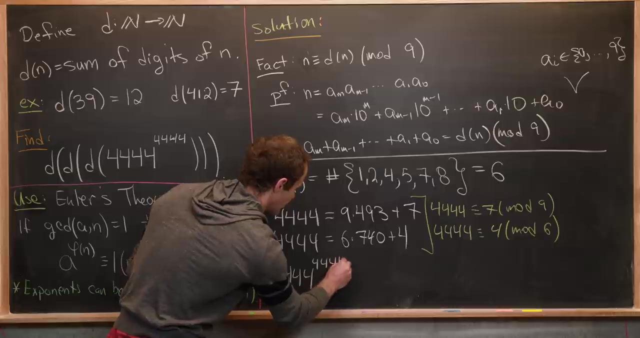 4, 4, 4 is congruent to 4 mod phi of 9, which in this case is 6.. But using Euler's theorem, along with just general properties of congruences, we have 4,, 4,, 4, 4 to the 4, 4, 4, 4 must be. 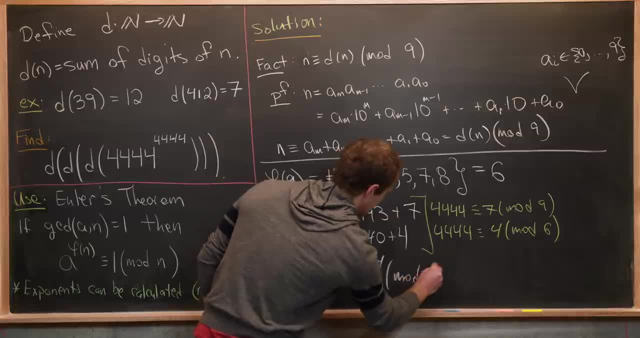 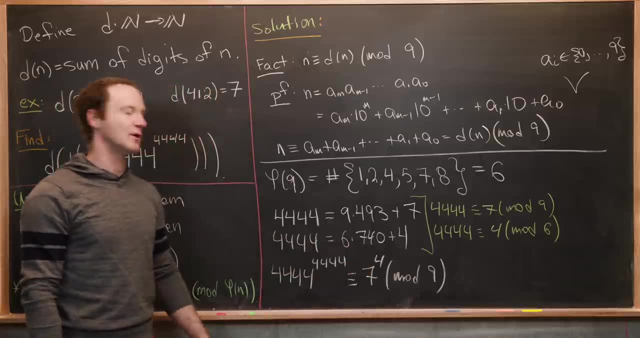 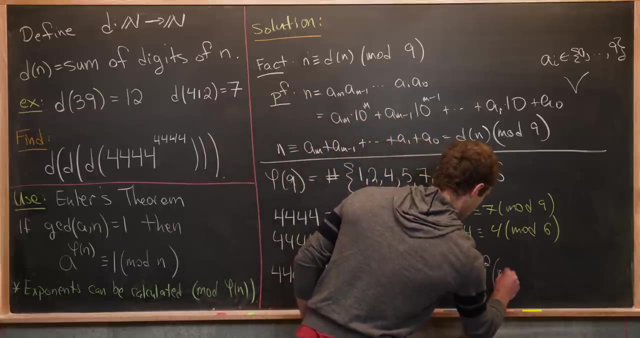 congruent to 7 to the 4 mod 9.. So notice we've reduced our base modulo 9, and we've reduced our exponent modulo 6.. But notice that that is going to be congruent to 49 squared mod 9, because 7 to 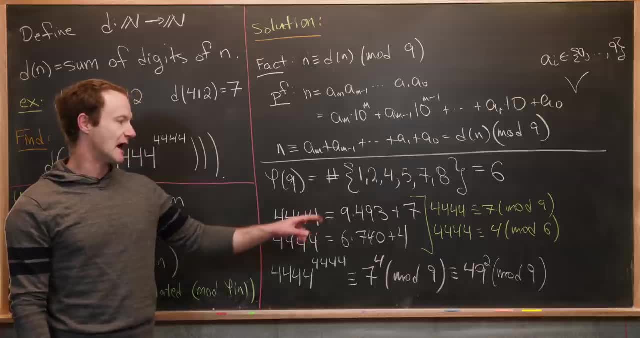 the 4th is just 7 squared squared. But now we can take 49.. But now we can take 49.. Notice that 49 is 4 mod 9.. And that's going to be congruent to 49 squared mod 9, because 7 to the 4th is just 7 squared. 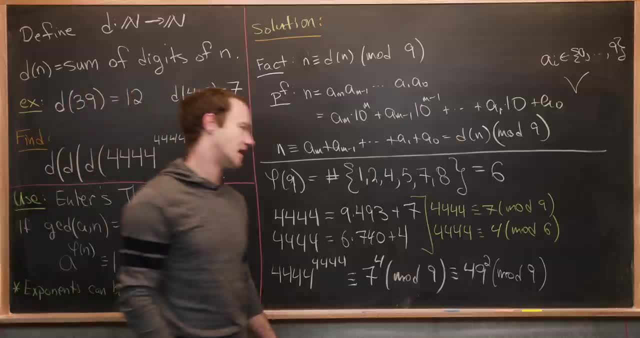 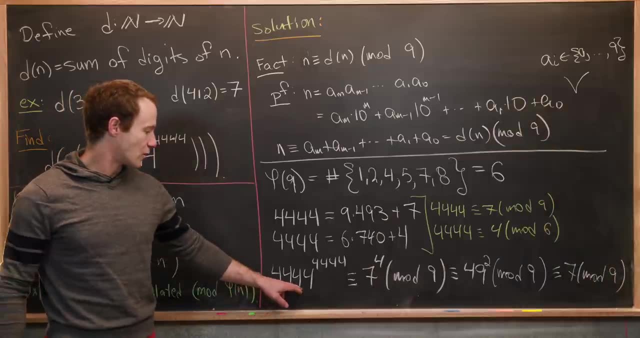 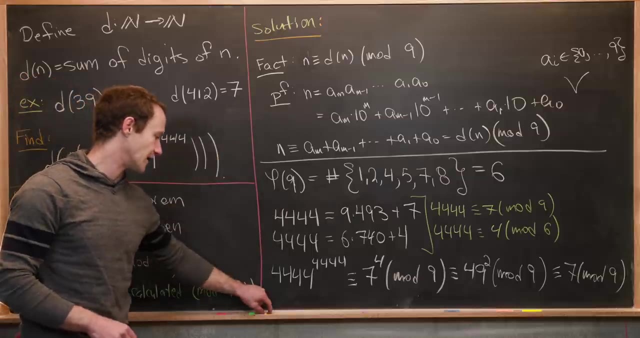 which makes 49 squared 16 mod 9, but 16 is just 7 mod 9, so we've got 4, 4, 4, 4 to the 4 4 4. 4 is congruent to 7 mod 9, but then, using our fact up here we have that. 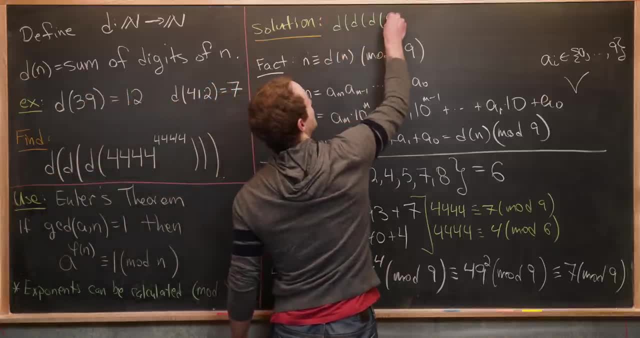 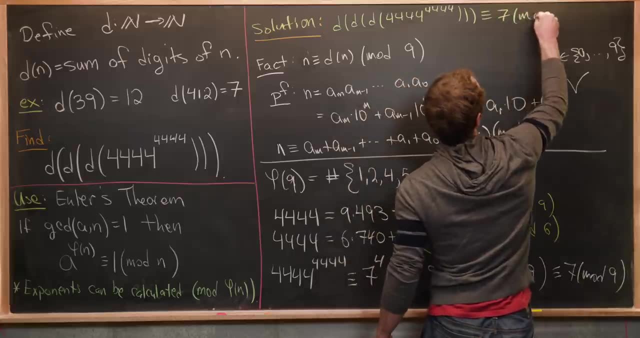 D of D of D of 4, 4, 4, 4 to the 4, 4, 4 4 is also congruent to 7 mod 9. okay, let's get rid of most of this calculation and we'll move on to the next step on the. 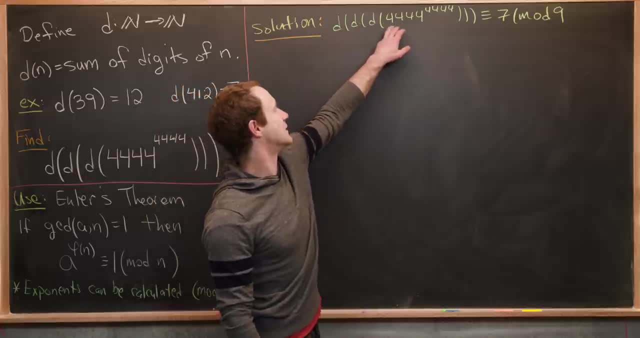 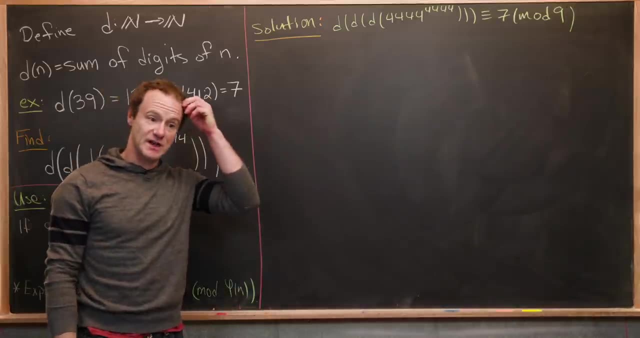 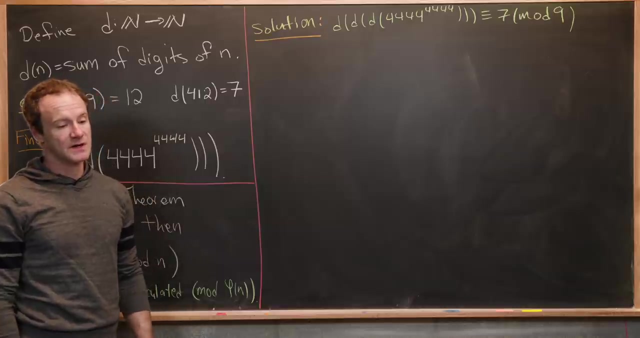 last board we determined that D applied to D applied to D applied to, our number was congruent to 7 mod 9. and now we're gonna use another trick involving logarithms to get some bound on the size of our goal number. so let's maybe look at this. 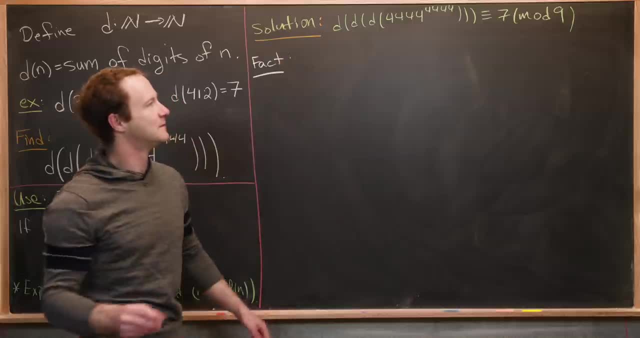 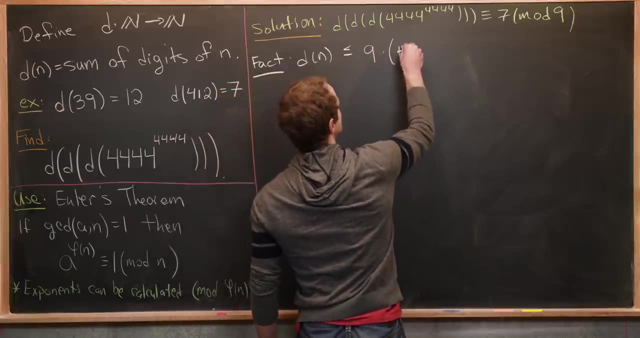 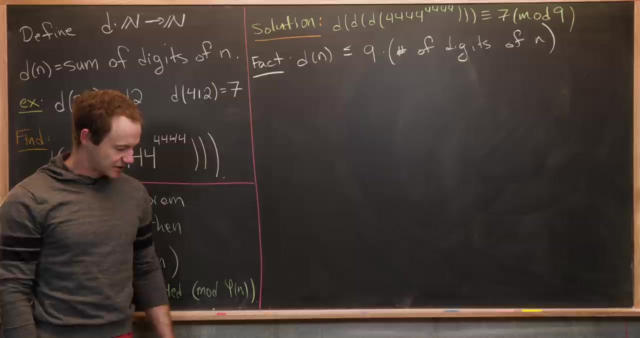 fact, kind of in parallel to what we had on the last board, and that is D of N is less than or equal to nine times the number of digits of N. so that's pretty clear because if you had nine, nine, nine, nine, as many times as the number 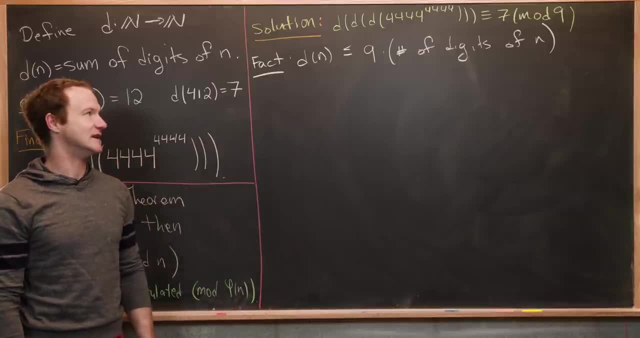 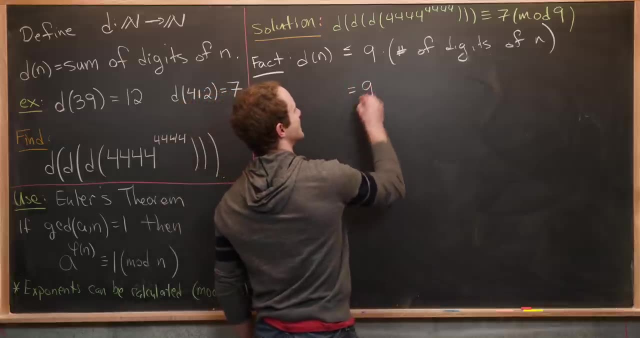 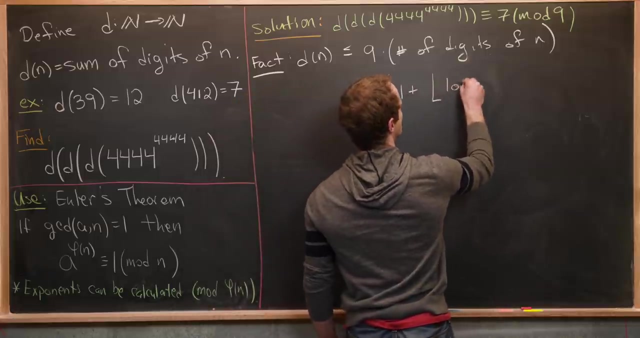 of digits of n, then you've like maximized this d of n. but now we want to write this number of digits of n in some sort of calculatable form, and the way that we can do that is using the logarithm base 10 and the floor function. so this is going to be equal to 1 plus the floor of the log base 10 of. 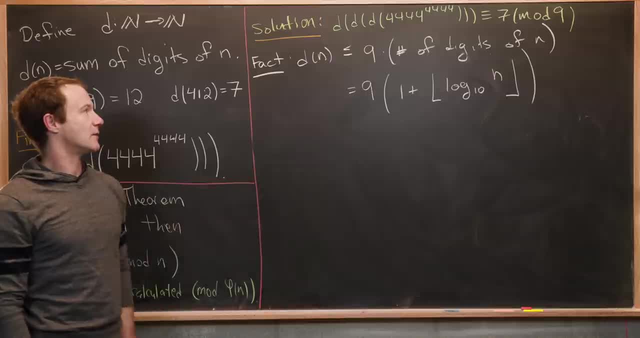 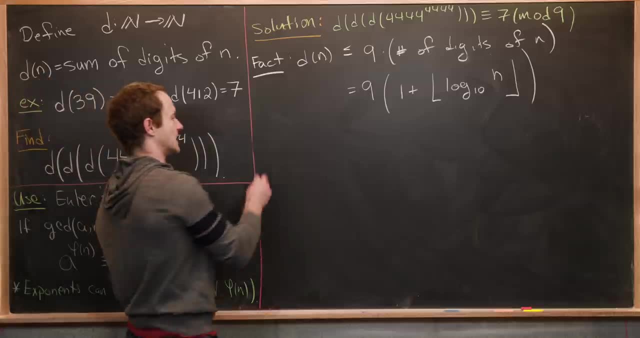 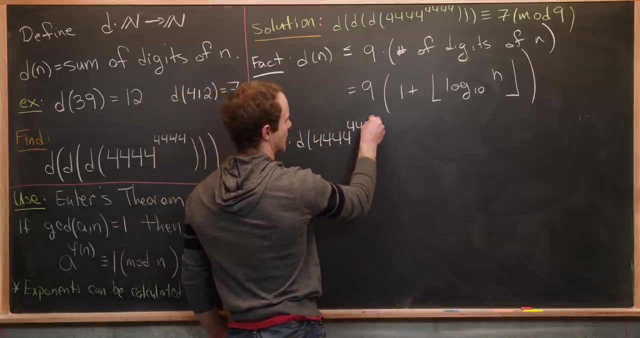 our number n. so now we can start applying this to our number: four four, four, four to the four, four, four, four. from the inside to the outside. so let's start from the inside. so d of four four, four, four to the four. four, four, four. maybe let's call this something for moving forward. so it's a little. 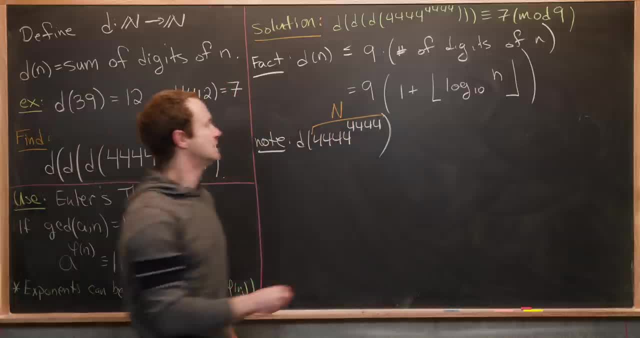 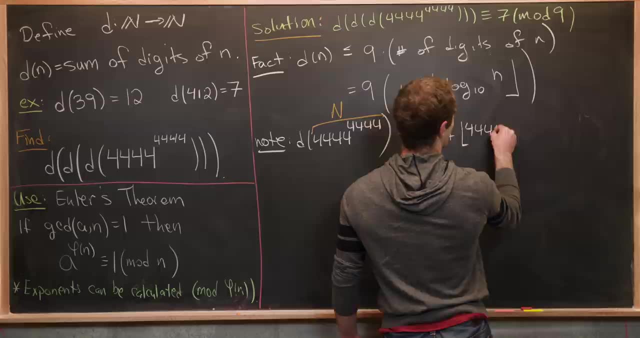 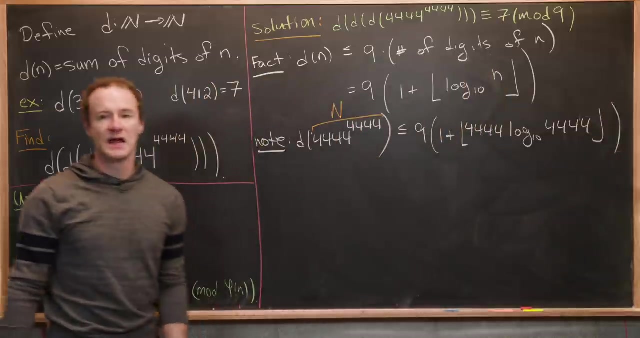 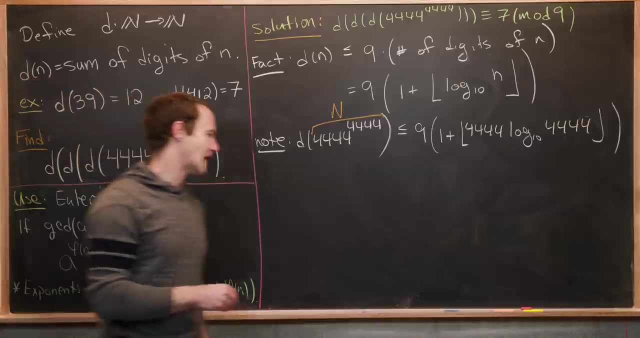 simpler. let's call this capital n, so that's going to be less than or equal to nine times one plus the floor of four, four, four, four. log base ten of four, four, four, four. great, and again that's using some logarithm rules involving exponents. okay, but now we can see. 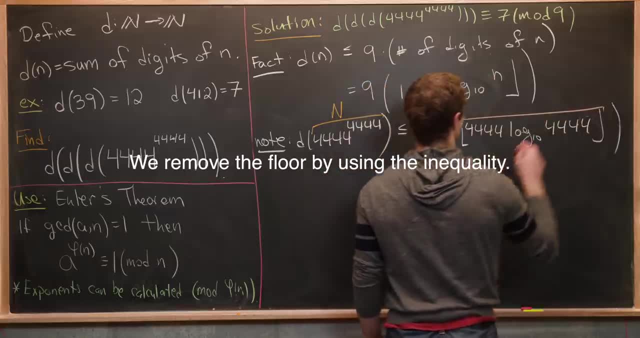 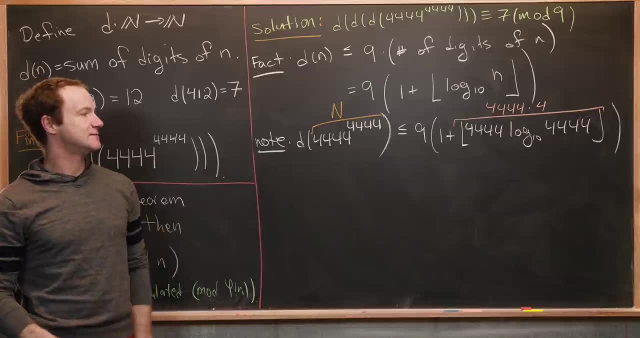 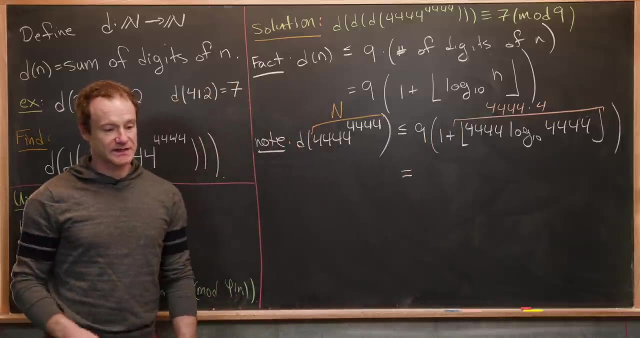 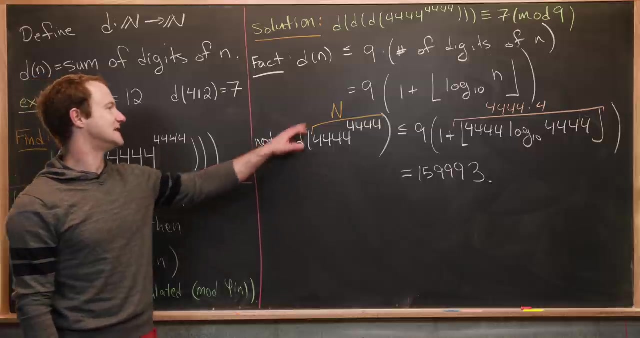 pretty clearly that this object right here will be equal to four, four, four, four times four. so now let's make that calculation and see what we get. so adding one to it and multiplying by nine, we see five, nine, nine, nine, three. so that means d of this capital, n is less than or equal to. 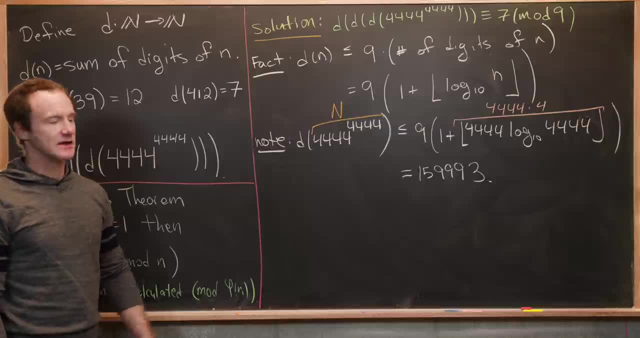 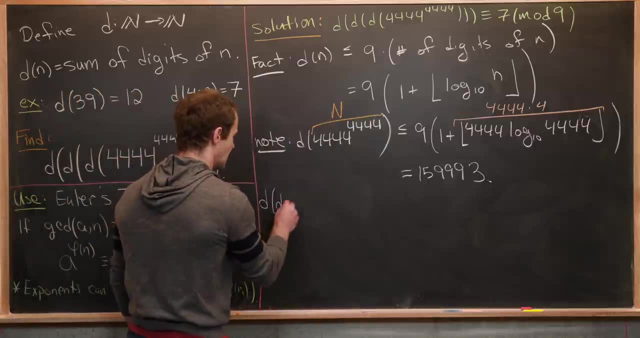 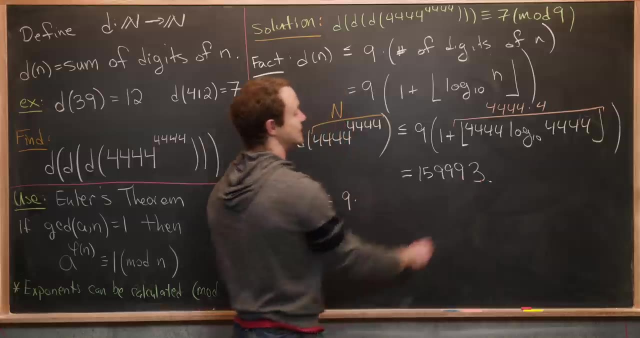 one hundred and fifty nine thousand nine hundred and ninety three. so now, working from the inside, outside again we'll calculate d of this object. so we've got d of d of n. so that's going to be less than or equal to nine times the number of digits here. so i won't use the logarithm because 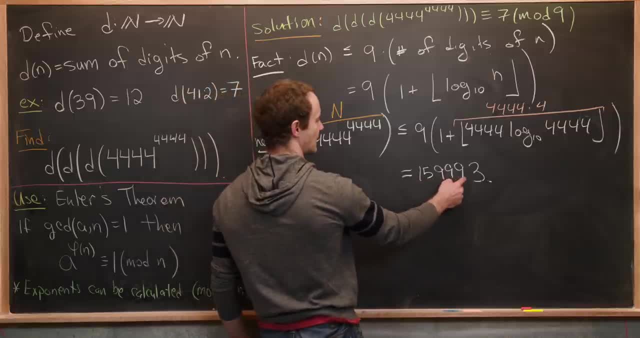 here we can just count up the number of digits. here we have two number of digits. we've got two, one, two, three, four, five, six. So we have d of d of n is less than or equal to nine times six. 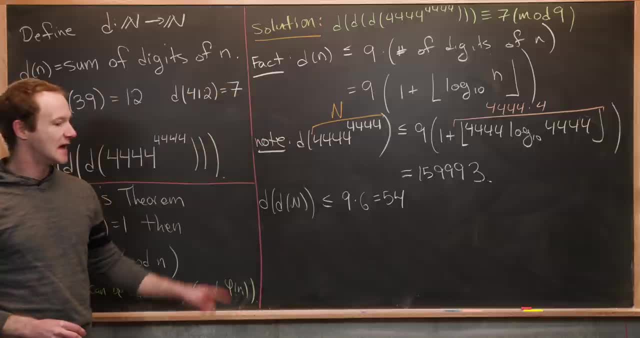 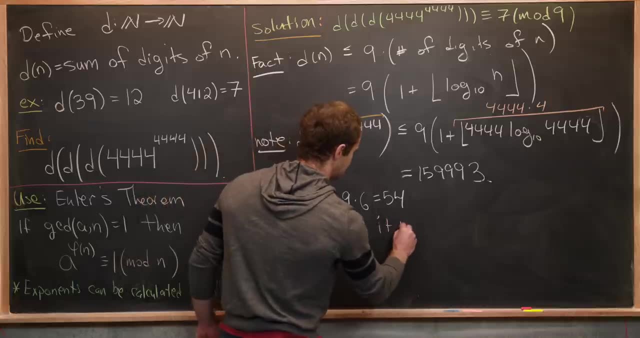 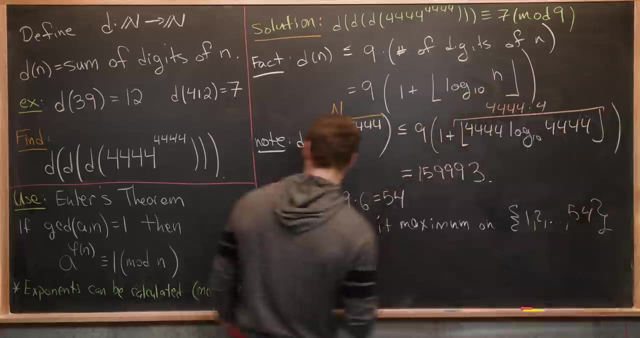 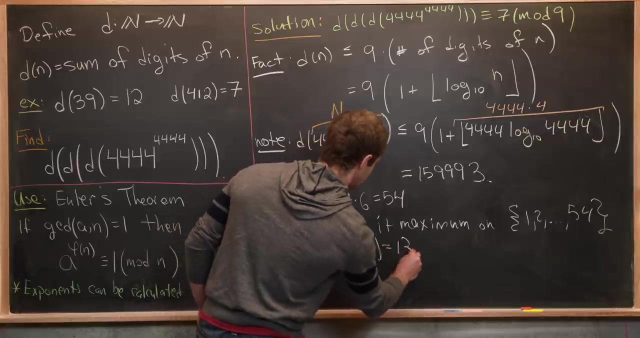 which is equal to 54.. And next, what we want to notice is that d of little n achieves its maximum on the set one, two, up to 54, at the number 49. And in fact, d of 49 is equal to 13.. 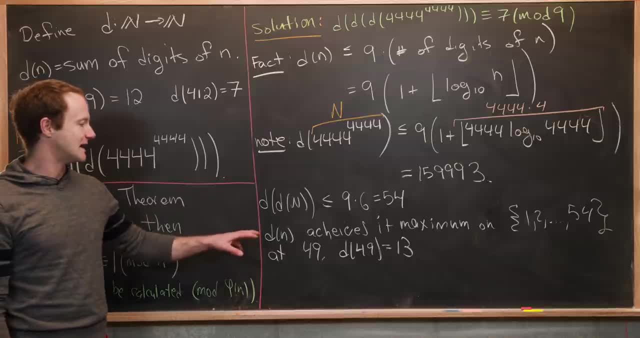 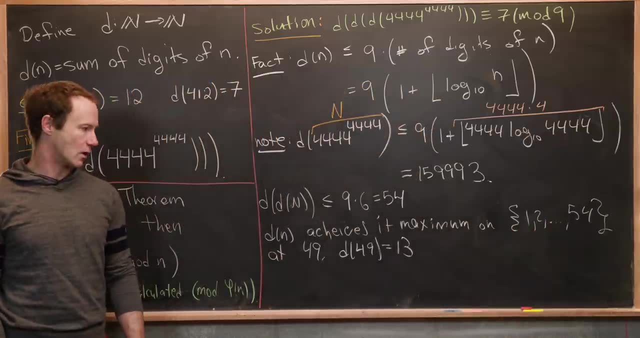 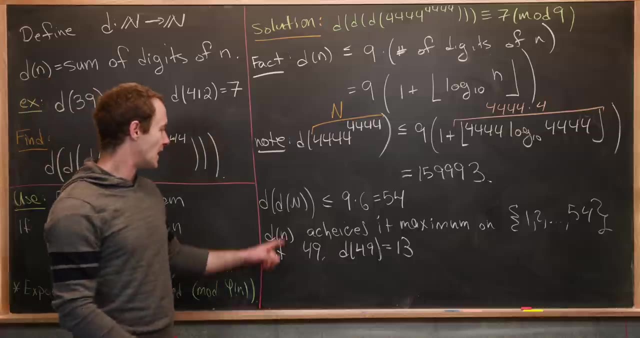 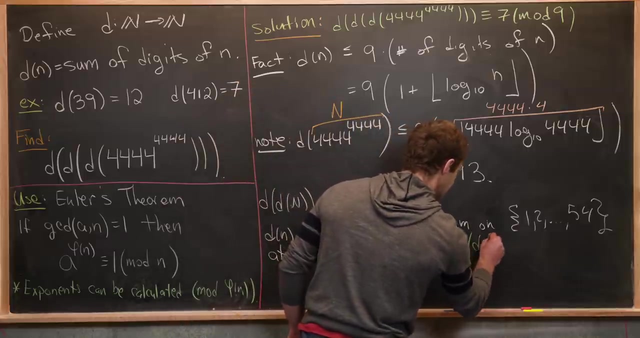 So what do I mean by that? Well, what I mean is if we apply d to any of these numbers, to one, two, three, four, up to 54,, then the largest output is 13.. Okay, But what that tells us applied to this rule up here is that d of d of d of n. 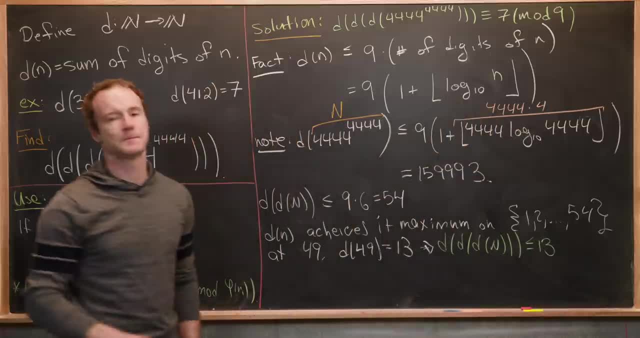 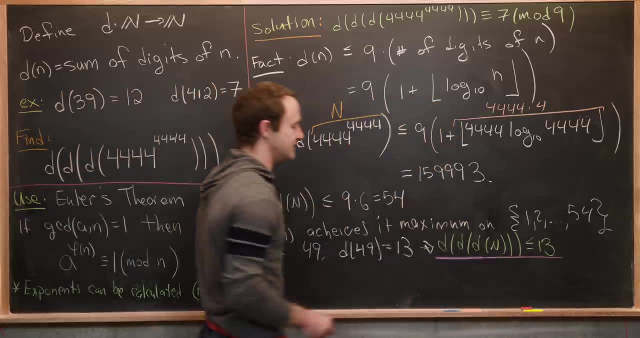 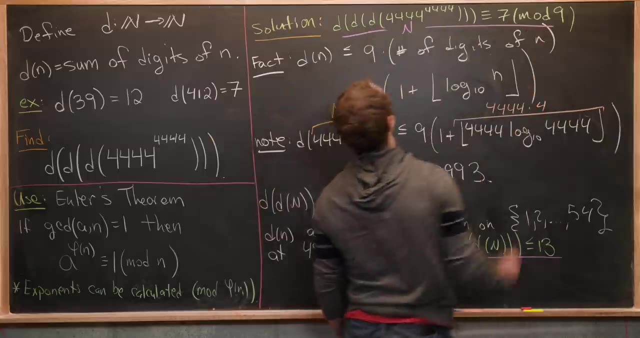 must be less than or equal to 13.. Okay, But now we have everything on the board that we need in order to solve the problem. We know that d of d of d of capital N is less than or equal to 13.. And we know d of d of d of capital N is congruent to seven.